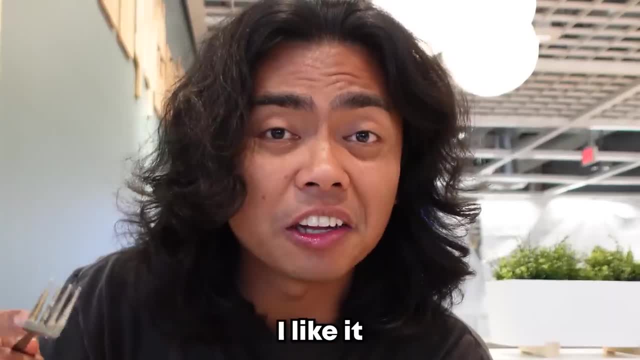 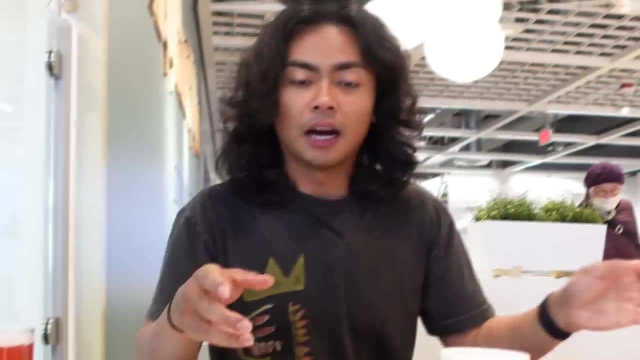 some syrup. it's good, i like it. i go with the syrup a little bit of lingonberry. i put it in the a tier. it's cool, i like it. if you combine it air tier, all right. moving on to the skagen croissant sandwich, okay, we have a little bit of shrimp. does it taste good? let's find out. 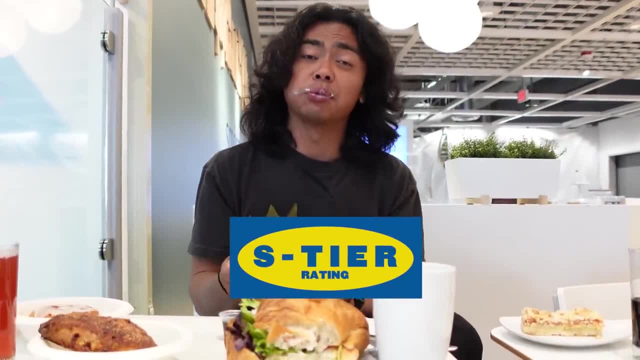 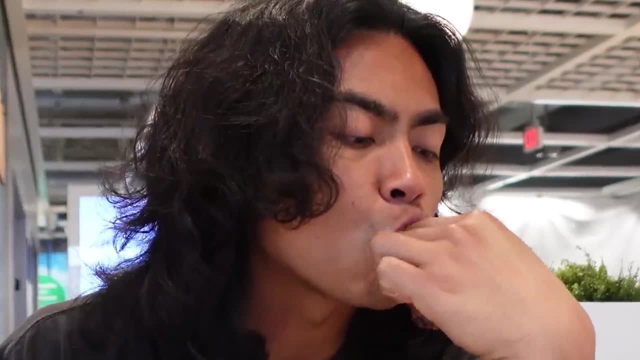 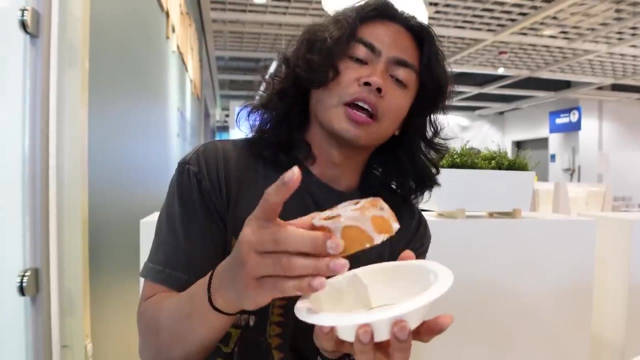 wow, okay, i like this. i'll put that in the s tier: breath coffee. um, this is the scone. okay, it's a little hard, it's kind of like rock candy. good, i put it in the b tier. okay, so this is cinnamon roll bruh. this is like my favorite pastry. 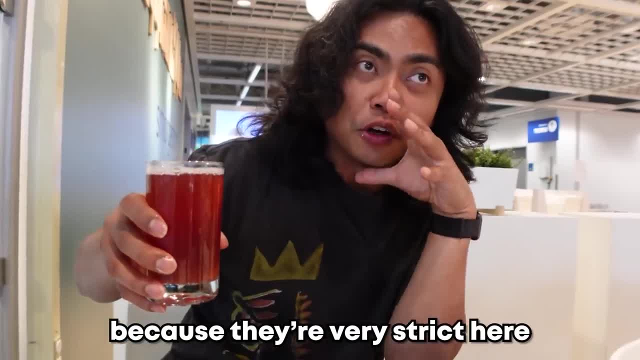 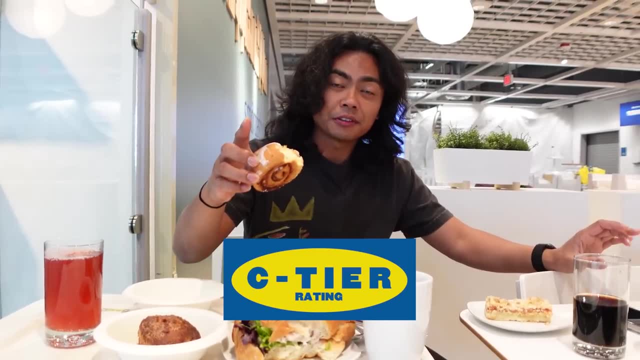 also, i gotta be a little quiet so we don't get kicked out, because they're very strict here and it gets. this is lingonberry, by the way. it's good. cinnamon roll c tier for cinnamon, lingonberry a tier. this is an apple strudel. 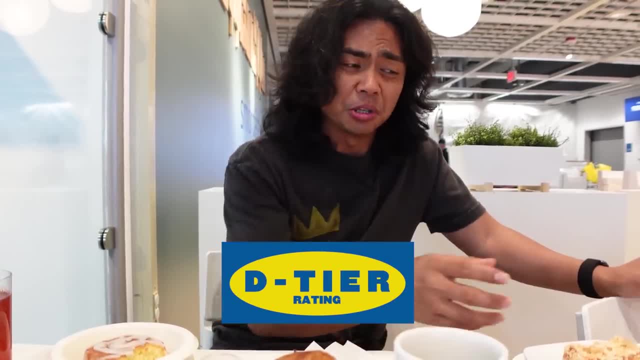 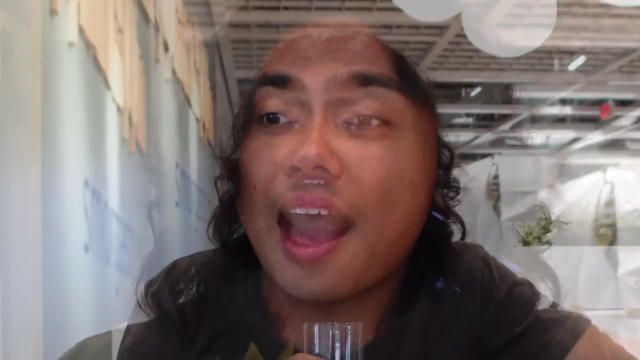 i don't like it. okay, i'll put that in like the d tier, just because i don't know this is so. this is a sparkling soda. ah, that's definitely c tier. it's like a bootleg pepsi. let's move over to the lunch portion. 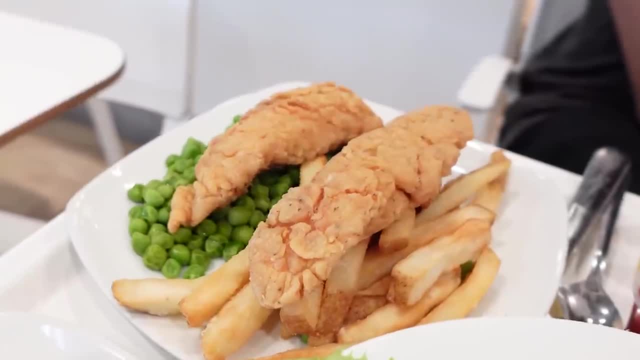 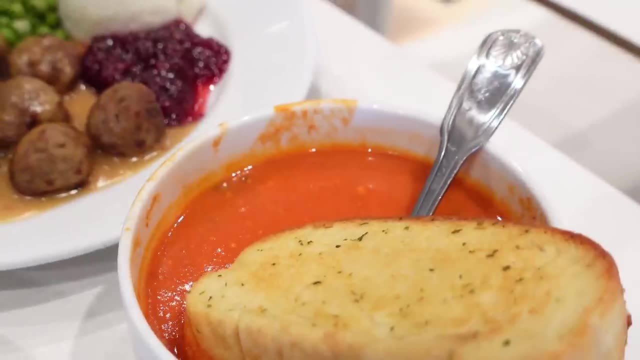 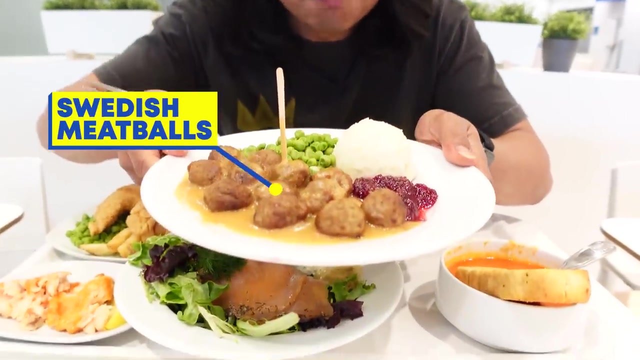 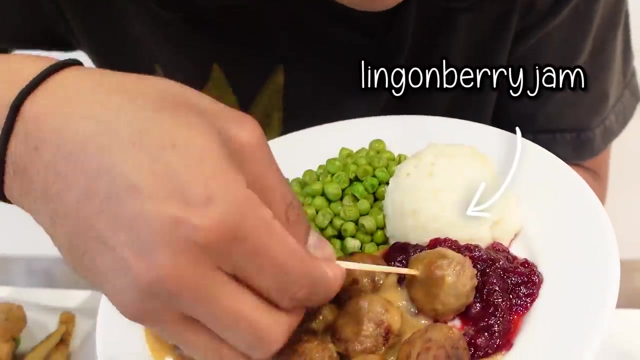 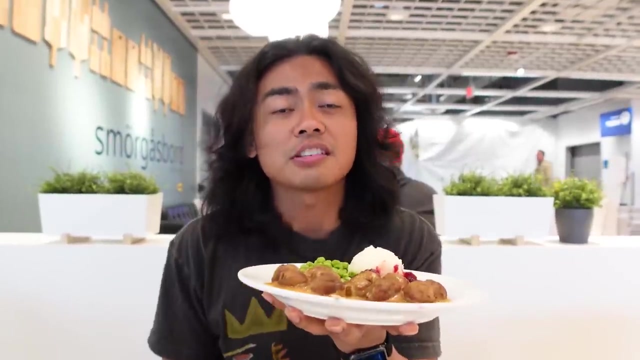 of ikea. this is the infamous swedish meatballs. what you want to do here is grab the swedish meatball, dip it in this little bit of gravy. dip it on the lingonberry jam sauce that are our also known as. this is delicious. put it in the ass chair just because there's a staple here. 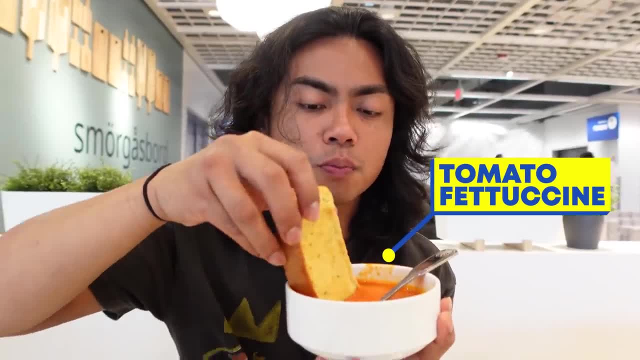 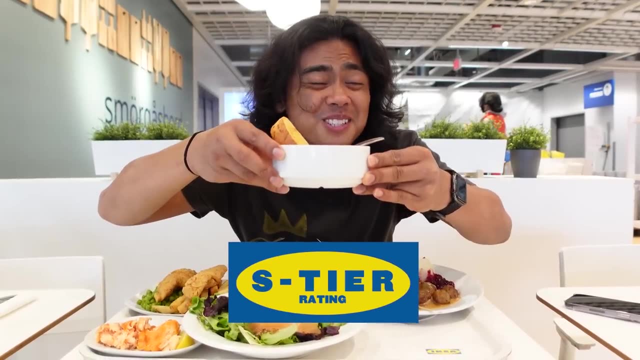 some might like it, some might don't. this is the tomato fettuccine soup. whoa the garlic bread. freaking bless up bro. this with the garlic bread s tier. this is pretty good. i love my soup and tomatoes. this is the stockholm salad, so let's try this. 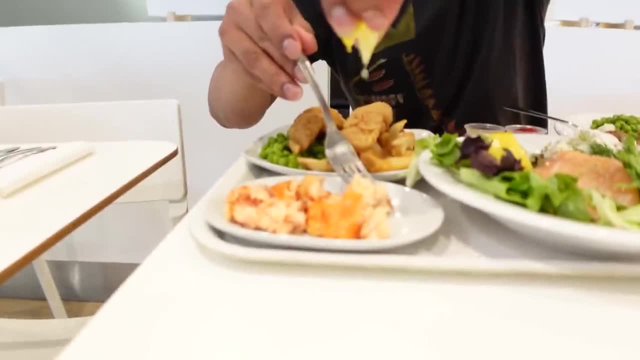 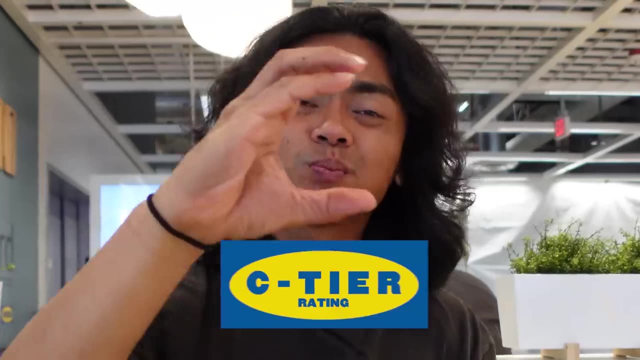 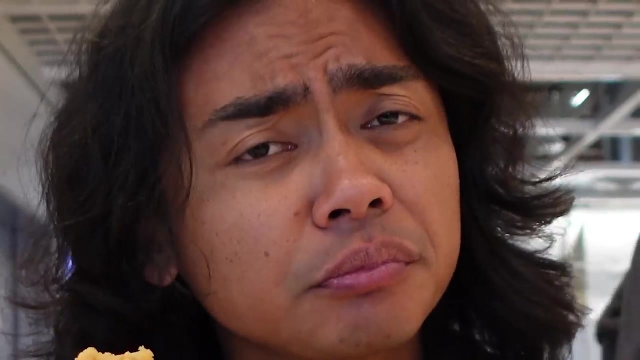 that's good. that was delicious. i'll put it in the b tier. this is hot salmon now, ah, a little dry. another popular item for the kids: they're chicken tenders. that's pretty dry, so this is probably like these here. this is all right, but i want to. 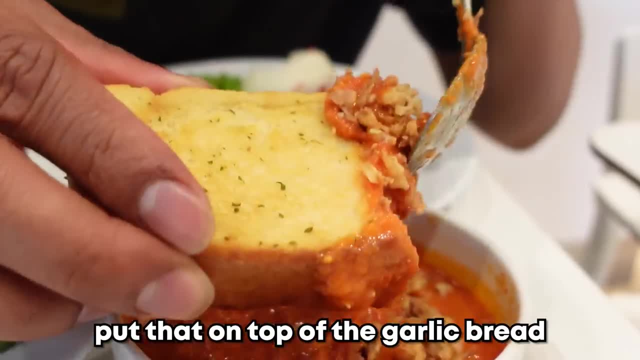 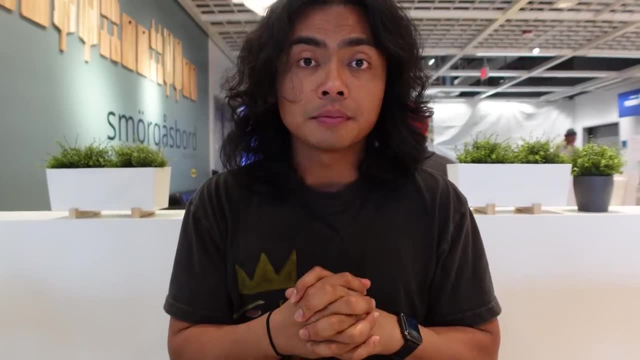 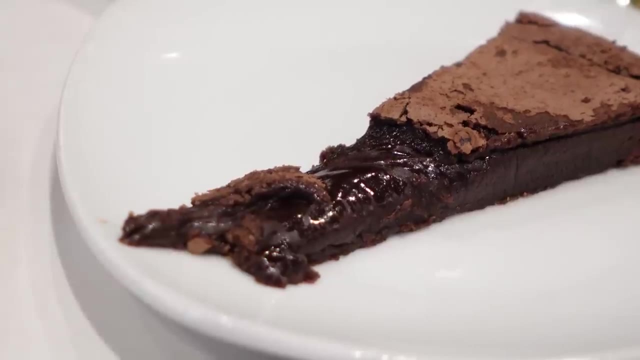 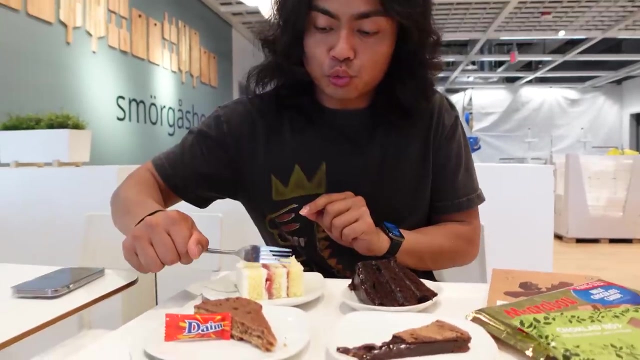 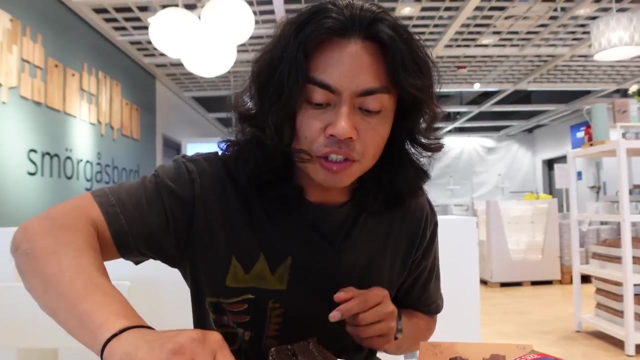 try to roast that. look, put that on top of the garlic bread. is that what i said? let's move on to some desserts. let's move on to some desserts. okay, we're gonna start with the strawberry shortcake. it's good, not too sweet a tier. this is the triple layered chocolate cake. 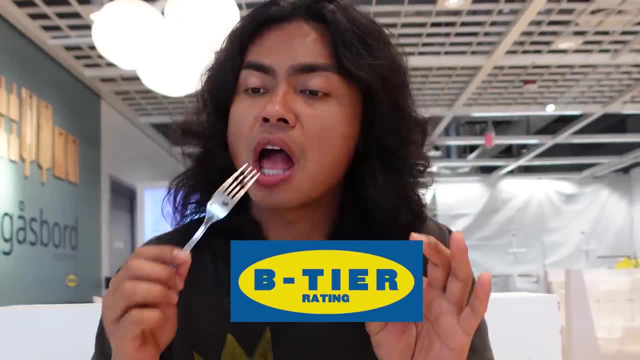 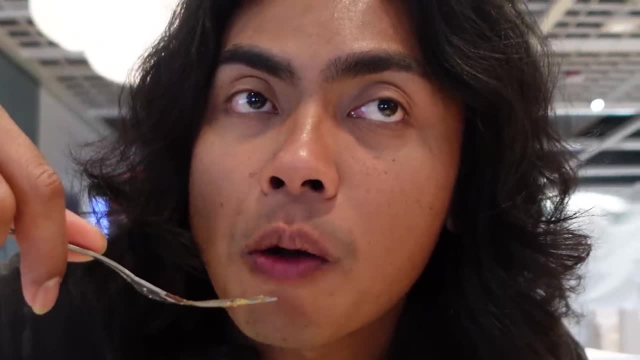 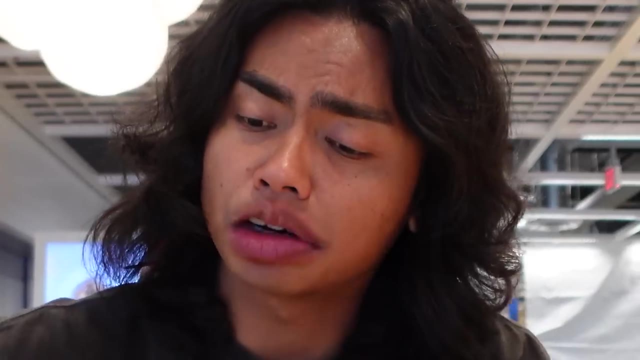 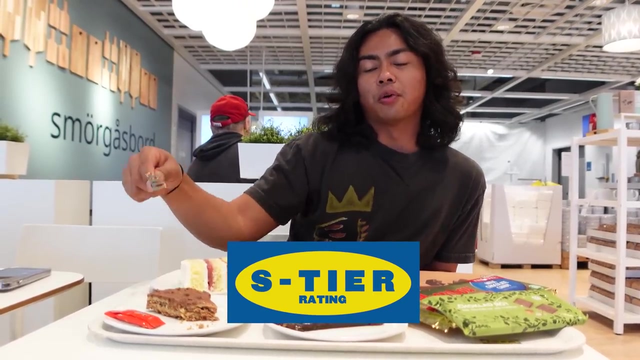 it's good. it's chocolatey, a little wet, but not that great b tier. this is their caramel almond cake. it's like so layered, it's pretty good. remind me of a kit kat coconut, coconut. you say caramel or caramel. that's great, great, like damn. this is good, that's here. this is like one of my favorites in here. i don't know why. 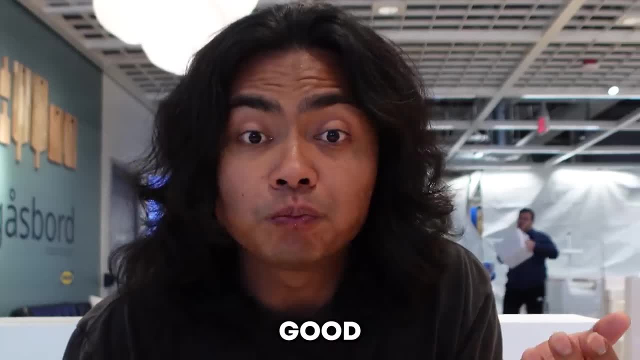 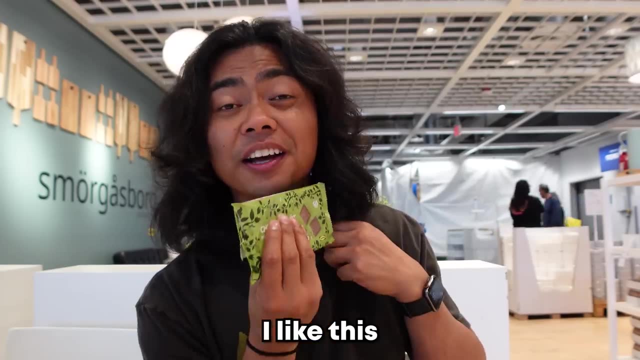 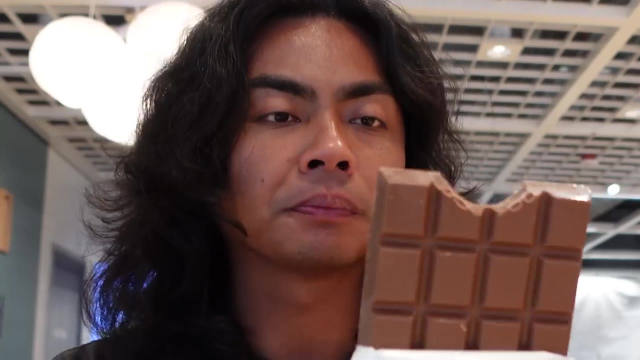 chocolate gooey cake. oh good, we're gonna try out their chocolate bars. okay, this is the chocolate nut. um, i like this. oh yeah, it's good. eight here. next we have mild burrow, pretty big bar. it's good, it's very plain. use ganaska day, okay. so i've been waiting to do this. the 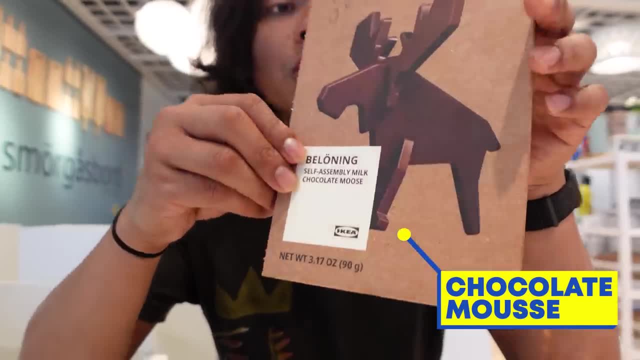 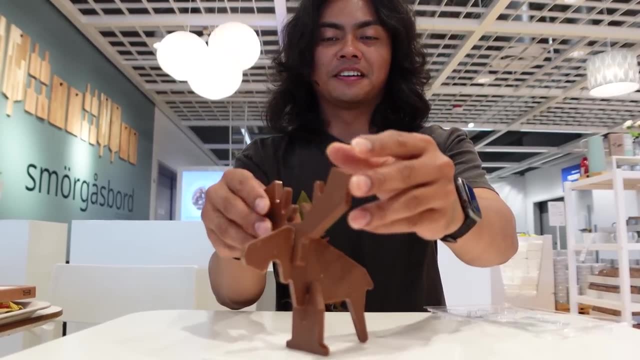 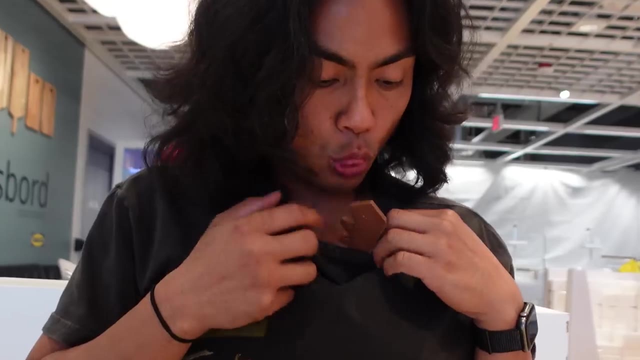 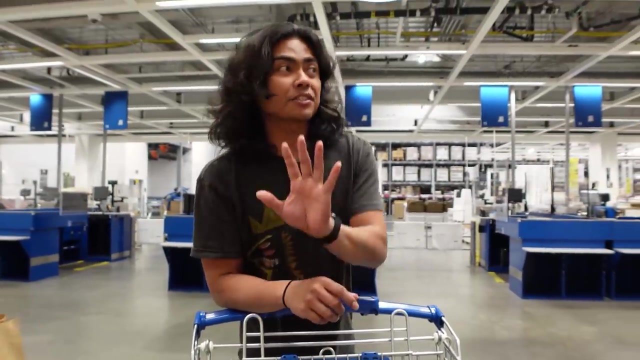 whole entire time. this is the chocolate mousse where you assemble it like legos. okay, step one, step two and you have yourself a ballooning. this is like double s tier: 100%. i don't even have to eat it, it's good. so what a lot of people don't know about ikea is there's a whole grocery aisle. 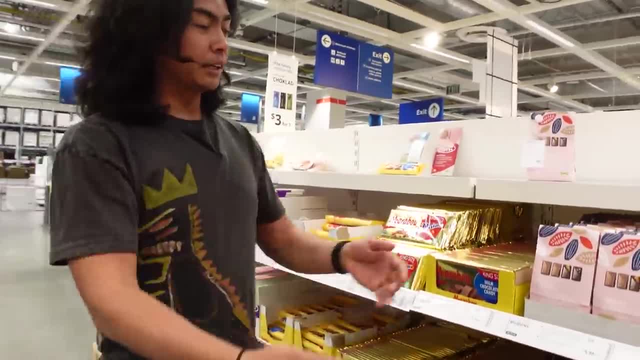 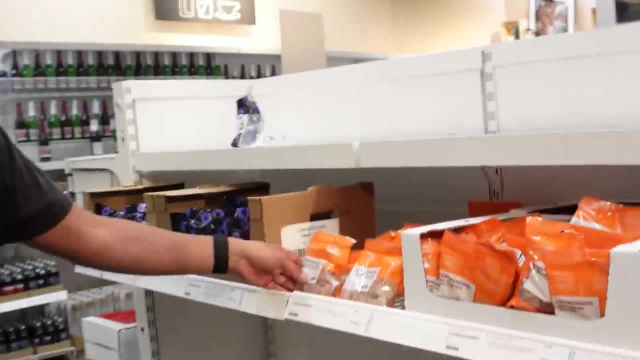 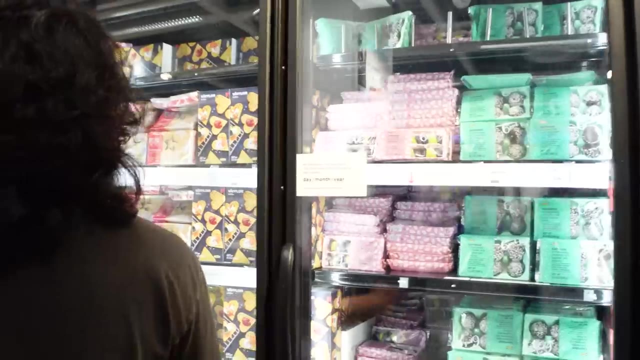 here where you get random snacks. so this whole area. there's a whole thing of dams, there's a, there's a marabou- damn, we got the kefir. they got so many lord gaga google zero. i guess lord gaga google just means like freaking squishiest, they have jacks. whoa, they got cute waffles. 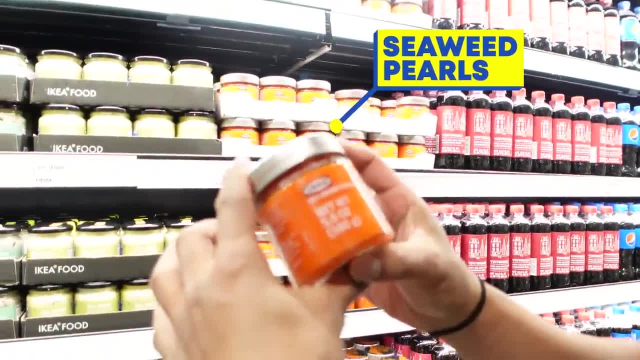 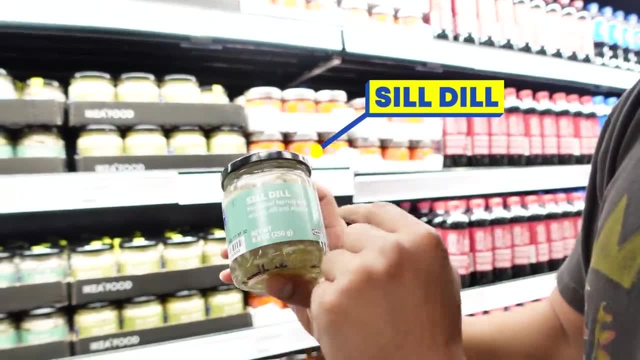 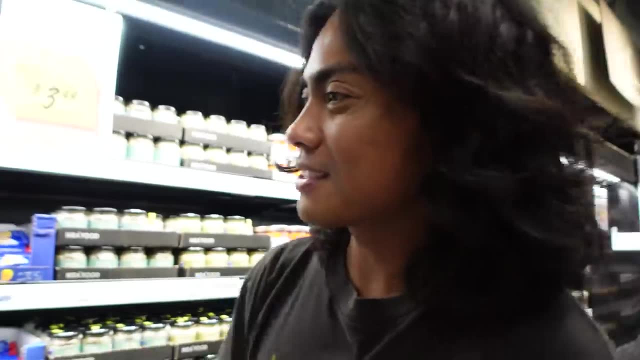 let's try it out. we got some red seaweed pearls. uh, it's just marinated herring and mustard sauce seal deal. this looks disgusting right here on the top, but i'm sure if you shake it it still looks disgusting. i'll take it, though. we have kales. that's so sick. 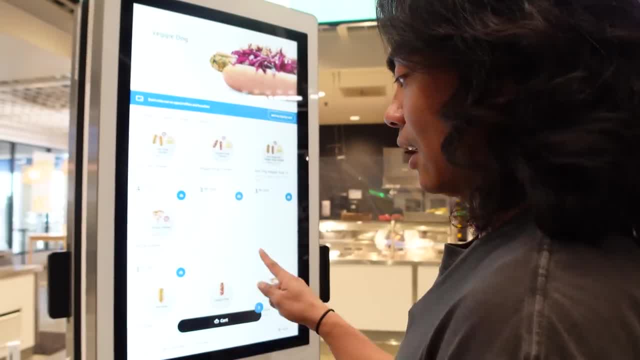 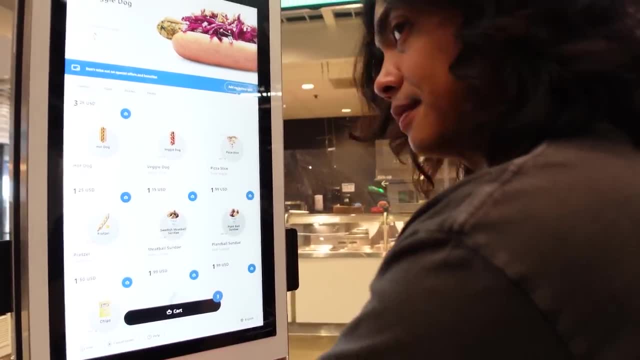 so it's very similar like costco, very equivocal. they have, like hot dogs, meatball sundae. i'll take a meatball sundae, i'm gonna scan all these things and, uh, let's eat some of these snacks. this is the swedish meatball sundae. all right, it's literally what we had earlier, if you want just. 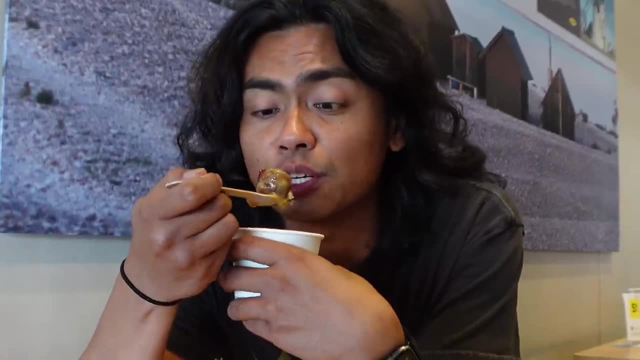 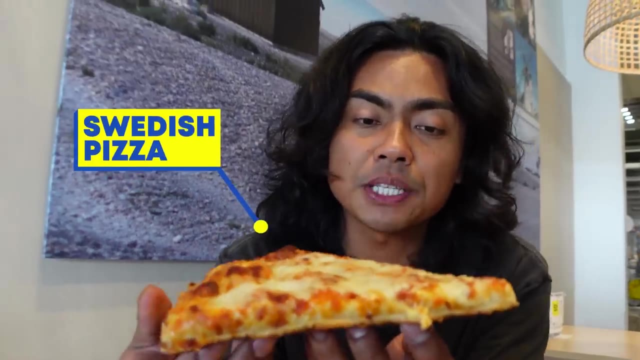 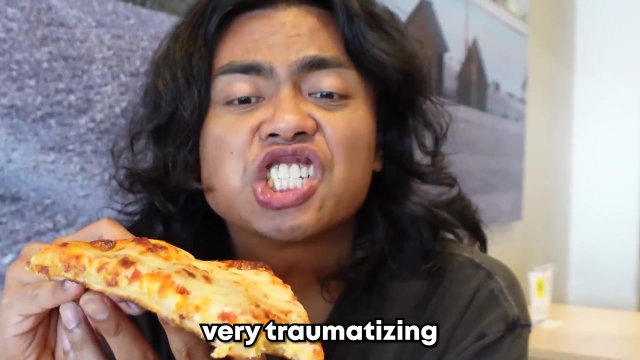 a good, good, simple snack. this is probably your snack to go to does the job. nice and warm, okay. swedish pizza looks like your uh, high school cafeteria type. it tastes like a two- very traumatizing. moving on, it's the first time where i saw the bun. the bun is not as big as you think. the bun is. 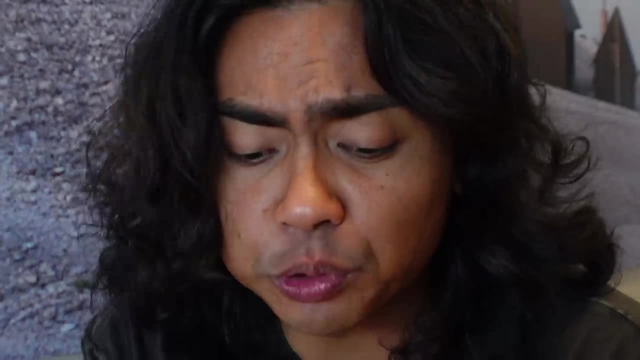 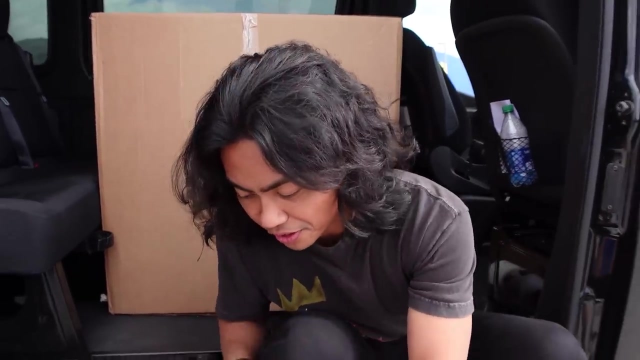 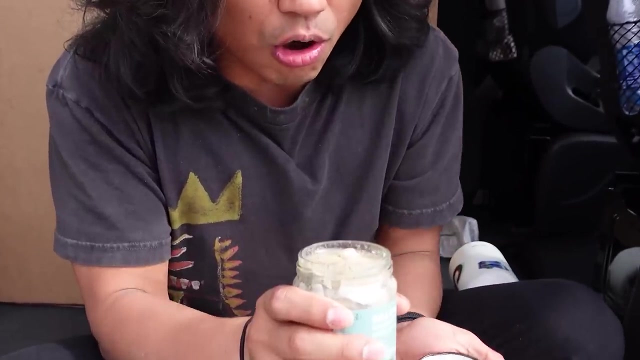 but it's really good. you know what that's good. i'm not really a hot dog guy, but good, all right. so we are here. uh, let's try out some of these snacks. okay, we're gonna start off with this nasty one. this: i don't understand what this is- seal dill. oh, my lord, oh. 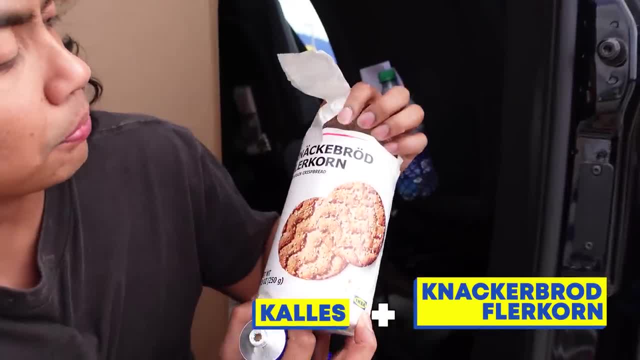 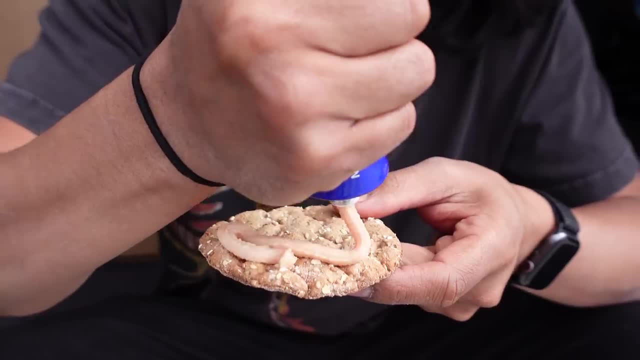 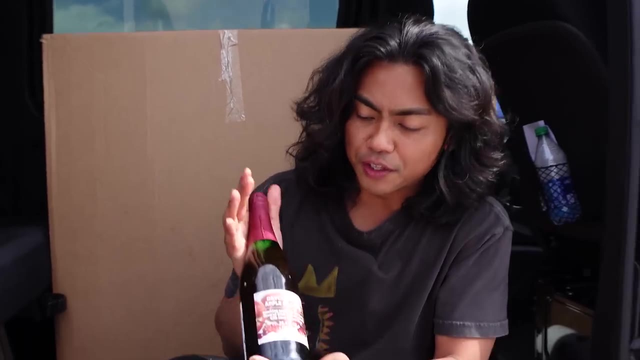 yeah, that's good, it just looks disgusting. okay, so let's take some of this um flair thorns and we're gonna slap a little bit of this toothpaste. this is just row, which is, i guess, fish, just like that. here we go. that's actually pretty good, wow. next up we have the. 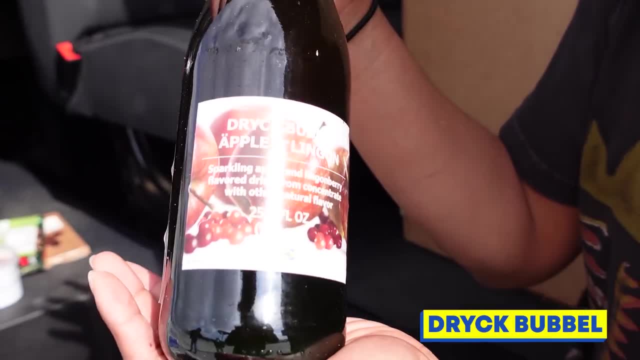 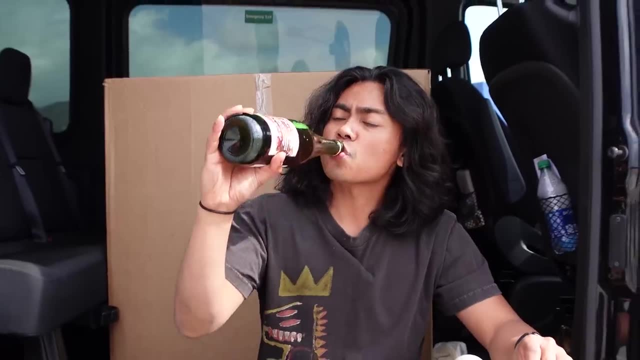 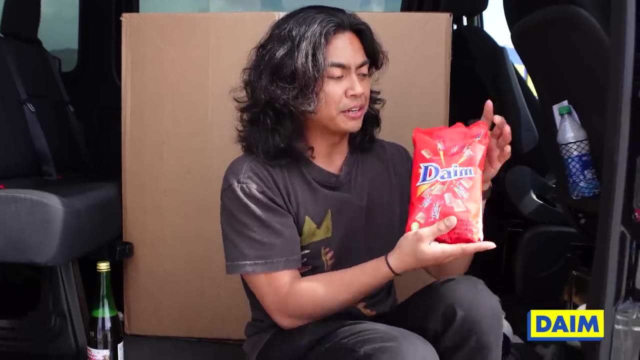 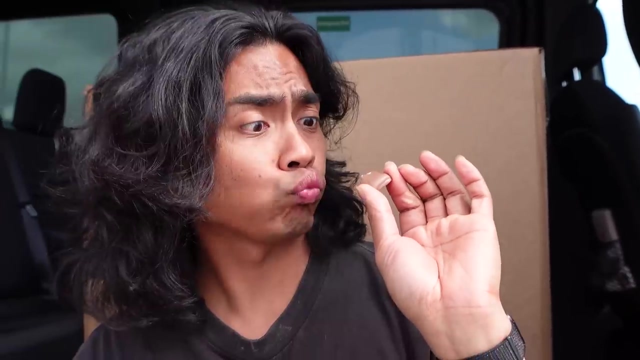 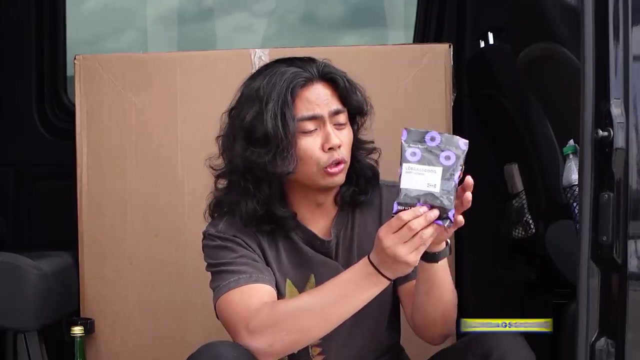 drake bubble. this is a sparkling apple and lingonberry uh flavored drink from concentrate. look at this. um, that's actually pretty refreshing. it's like a cidery. all right, so we saw this earlier. we're going to go with the. so this is a like a chocolate cake. it's like a cake with the sugar on the bottom. 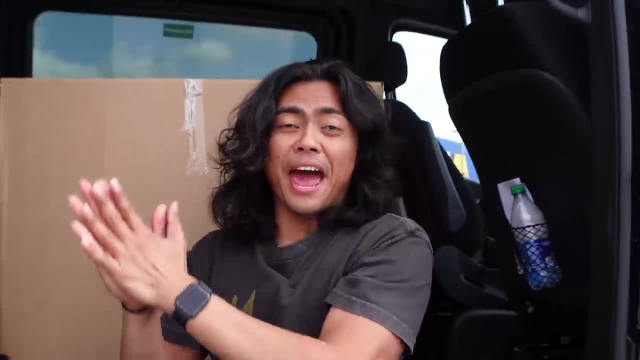 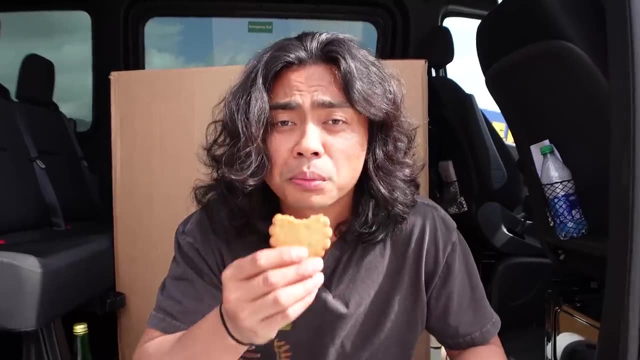 and then it's just like a, like a cake cake. these are just damns like damn nice. you can tell it's gonna be quite a hard candy. it wraps around my palate like shakespeare. It's good. Okay, what is this? I want to know what kex is. Oh, they're little.